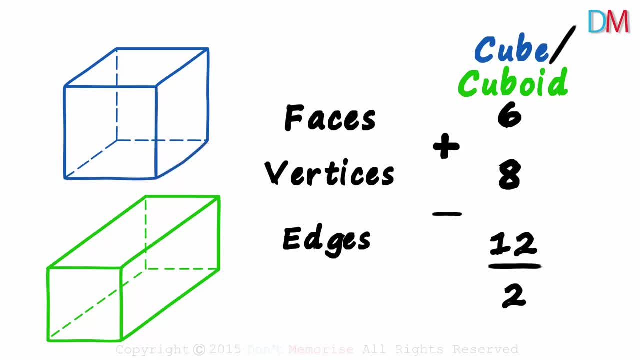 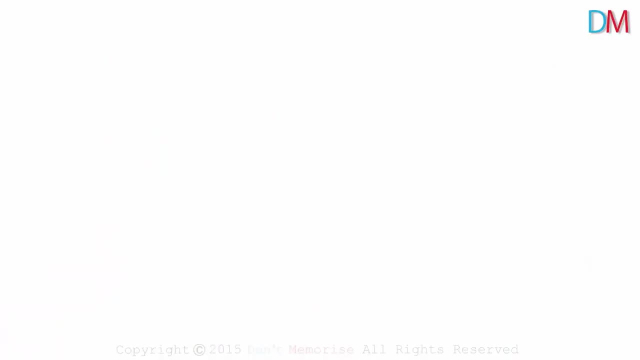 where the length, breadth and the height are equal. So a cuboid also has six faces, eight vertices and twelve edges, And F plus V minus E will give us two. Let's see if it works for other straight face solids. Do you remember what a square pyramid looks like? 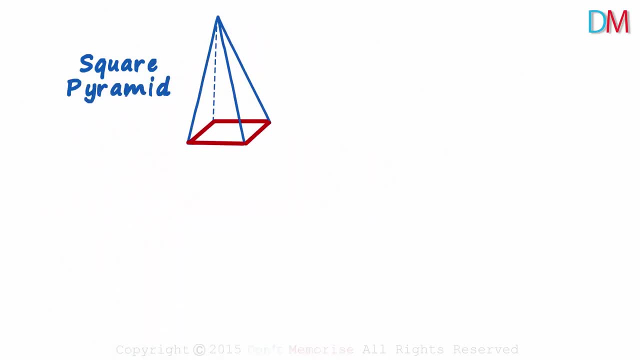 It is a figure with a square as its base and triangles as its faces. Square base and four triangles as faces. And what is a triangular prism? A prism is a three-dimensional solid which has identical and parallel ends and all flat faces. A triangular prism would look like this: 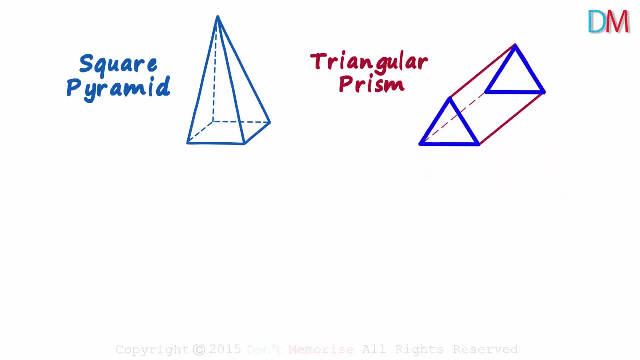 It has two identical and parallel ends. It has two identical and parallel triangles at its ends and three rectangular faces. What do we need to find out here? We need to find the number of faces, the number of vertices and the number of edges in each of the solids. 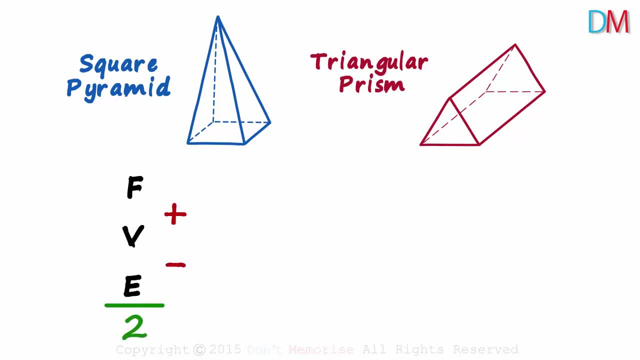 and see if F plus V minus E will give us two. Okay, let's tackle the first. solid, a square pyramid. How many faces do you see? There are four triangular faces and one square face. Five in all. How many vertices? 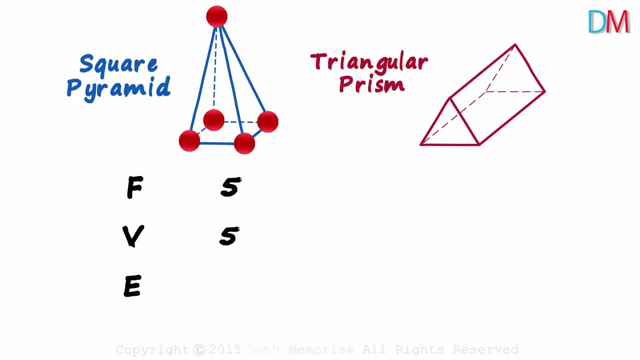 One at the top and four at the base. Five vertices And how many edges? Four slant edges and four edges at the base, A total of eight edges. We got F, V and E as five, five and eight respectively, And five plus five minus eight will give us two. 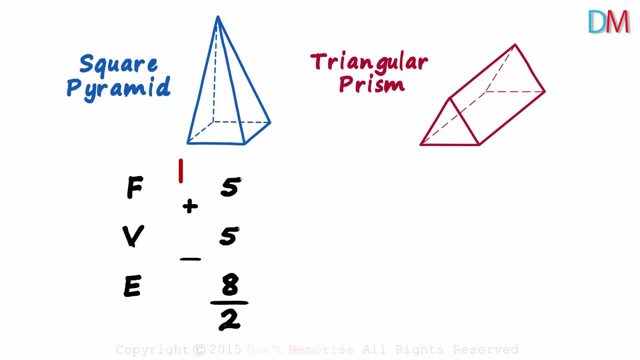 So it worked for the square pyramid too. F plus V minus E gave us two. This is called Euler's formula. For any straight face, solid F plus V minus E will always give us two. Will Euler's formula work for the triangular prism too? 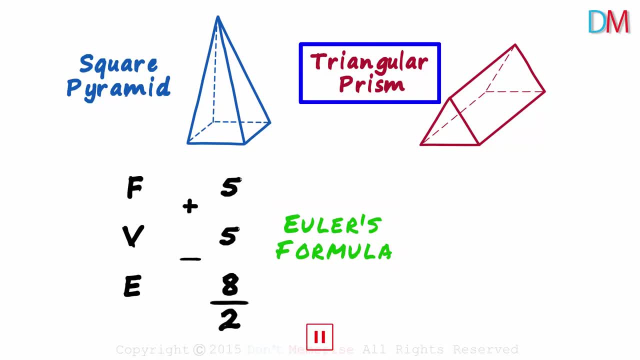 Why don't you give it a try? Okay, so how many faces? Two triangular faces at the ends and three rectangular faces in between. Five faces, How many vertices? Three at this end and three at the other. Six vertices: Three edges at the front face, three in between and three at the back face. 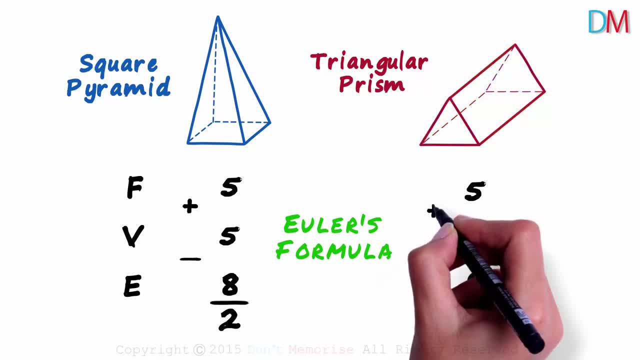 Nine edges in all, What will be? five plus six minus nine? Yes, we get a two, We will always get a two. That's Euler's formula: F plus V minus E will always give us a two, We will always get a two. We will always get a two. 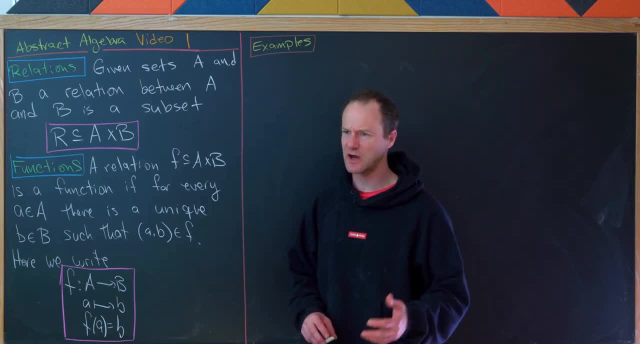 This is the first video in a series devoted to abstract algebra taught at the junior or senior undergraduate level. That is the last two years of university, but pre-grad school. 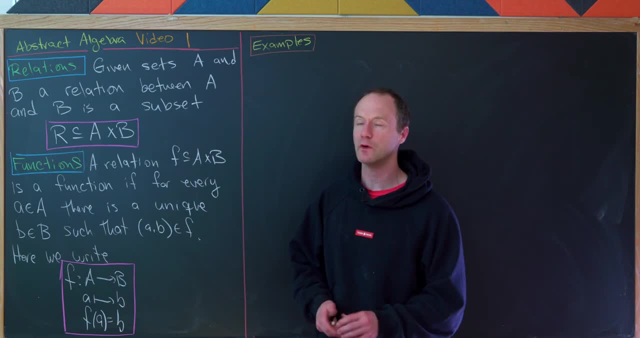 And today's video, as well as the second video, will be mostly devoted to reviewing some material that would come in an Intro to Proofs class. We'll move quite quickly through this material though, so if you need a bigger review you can seek that on on your own. I in fact have a 24-video series on Introduction to Proofwriting that will cover all of this material that we'll see today and much much much more in depth if you'd like to check that out. 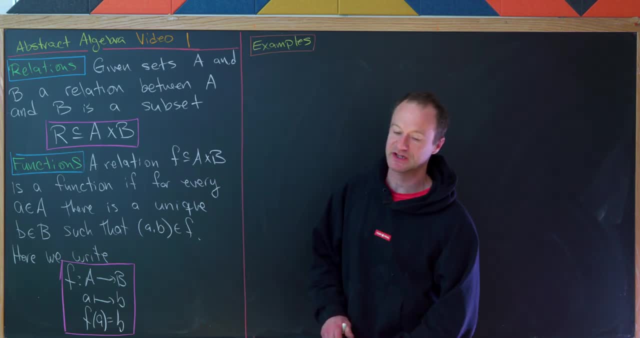 Ok, so today we're mostly going to be looking at relations and functions. So let's first look at a notion of relation. 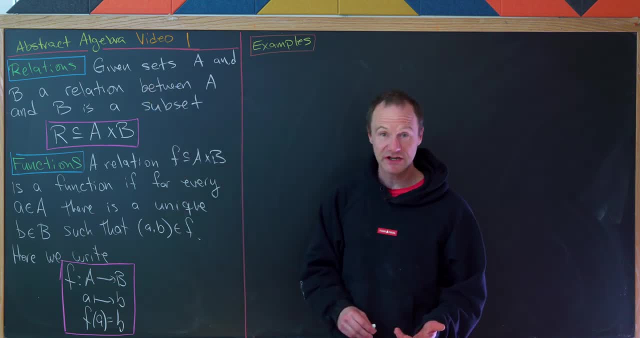 So given sets A and B a relation between A and B, That's b and c. So given sets A and b a relation between a and b a relation between a and b and b a relation 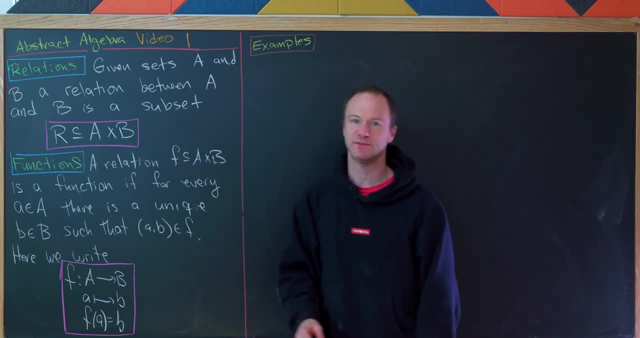 a and b is a subset of a cross b. So that's simply all you need for it to be a relation. 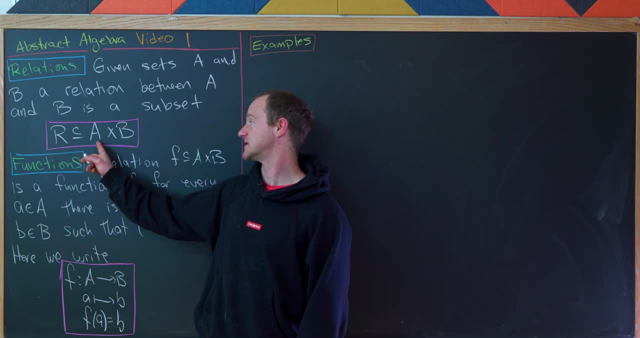 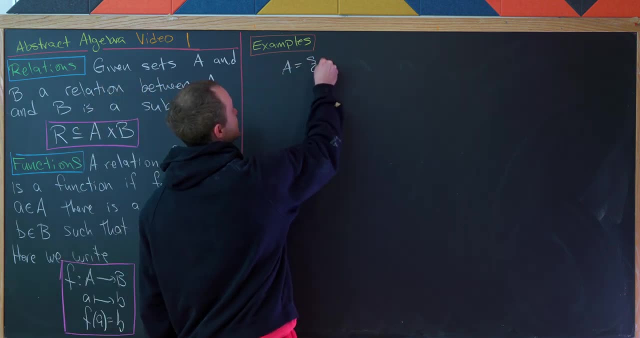 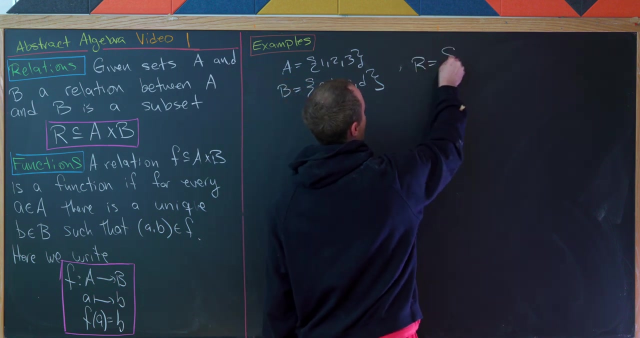 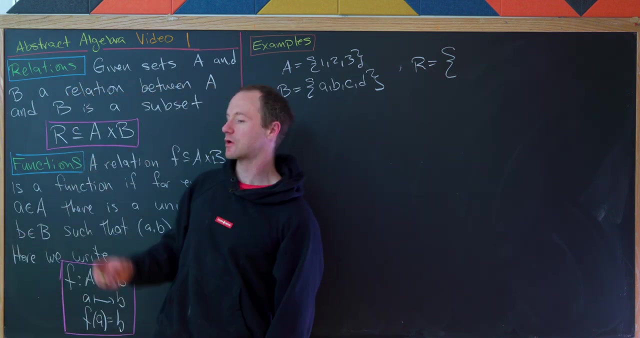 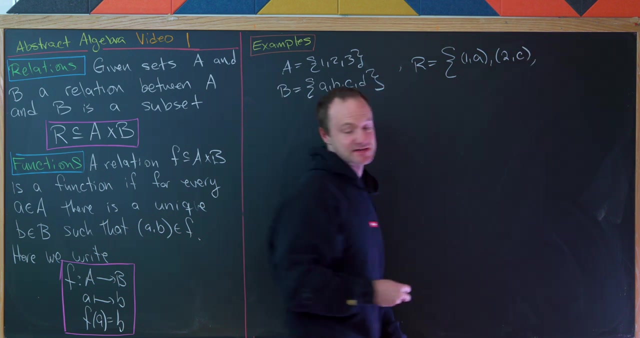 So notice I've written the relation as r. Like I said, it's a subset of a cross b. So let's look at an example of that. So let's take our set a to be the set containing 1, 2, 3. And let's take our set b to be the set containing a, b, c, d. Then we'll take the set r, which will be made up of ordered pairs, the first entry from a and the second entry from b. That's what we mean by the cross product here. And here we'll have 1, a, and then we'll have 2, c. And then next we'll have 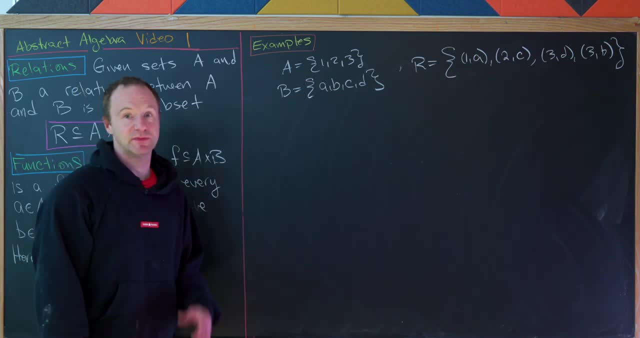 b. So that's most definitely a subset of a cross b. So that makes it a relation.